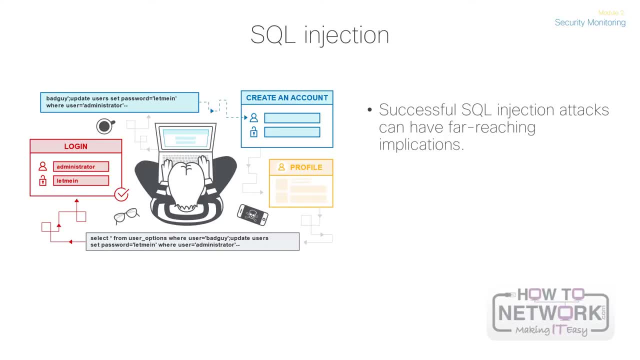 occurred back in 2012, when a hacking group collected the email credentials for 450,000 users using an SQL injection attack against an unnamed Yahoo subdomain. SQL injection attacks can be used to bypass authentication, disclose confidential information and distribute malicious code. 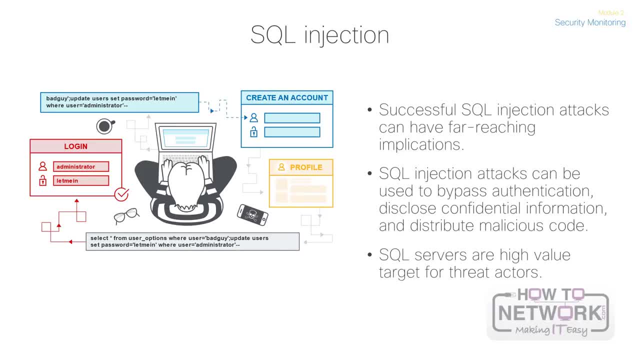 This makes SQL servers a high-value target for threat actors. The SQL injection attack uses attacker-supplied data to alter web application SQL statements. Unless an application uses strict input data validation, it is vulnerable to this attack. In fact, the Open Web Application Security Project lists it as the number one threat. 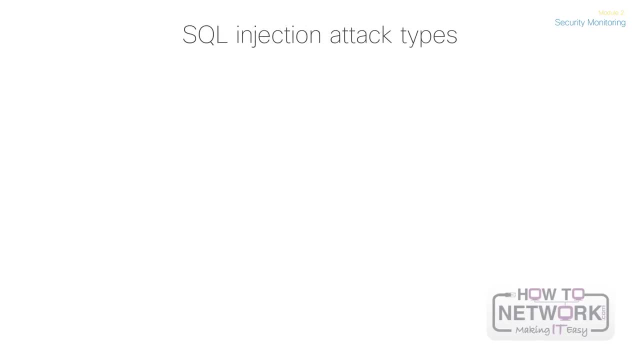 to web applications. Now let's look at some various SQL injection attacks. First is Authentication Bypass: Here it allows an attacker to log onto an application without supplying a valid username and password. Next is Information Disclosure: Here it is used to obtain sensitive information from. 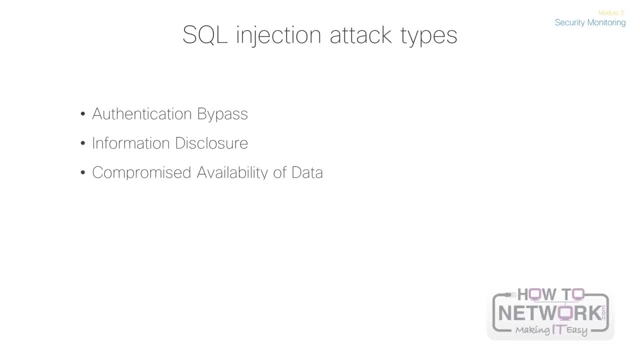 a database. Third is Compromise Availability of Data. Here the compromised data integrity involves altering the contents of a database to either deface a web page or insert malicious content. Compromise Availability of Data allows an attacker to delete information to either cause harm or delete log and audit information. 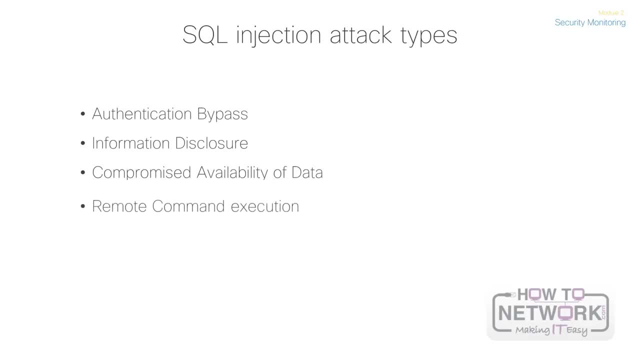 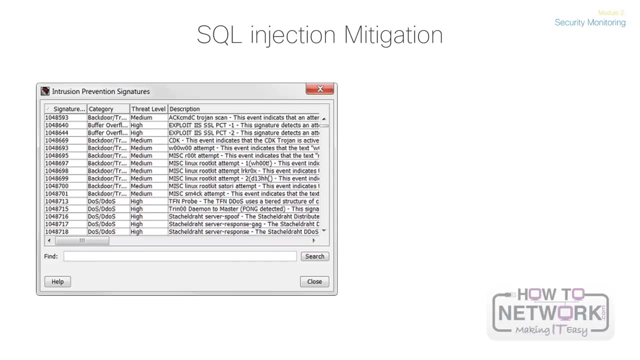 And finally is the Remote Command Execution. Here, it allows an attacker to compromise the host operating system. Now let's talk about how to Mitigate SQL Injection Attacks. First. let's talk about how to mitigate SQL injection attacks. First. let's talk about how to mitigate SQL injection attacks. 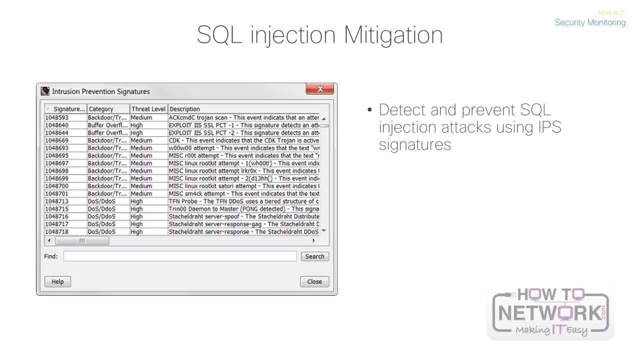 Intrusion Prevention System, or IPS, signatures can be used to detect and prevent SQL injection attacks, as long as it has visibility into the application traffic. End-to-end encryption, with HTTPS, for example, hinders the ability of the IPS to spot the signatures of the attack.